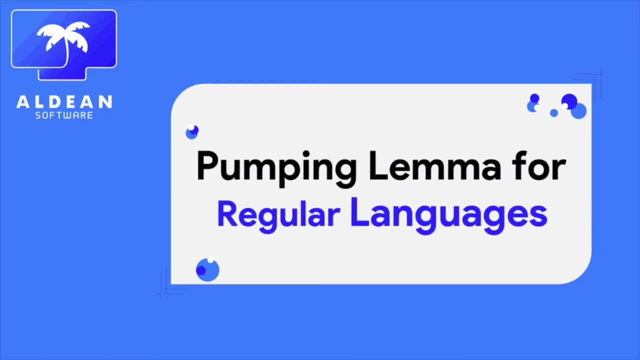 The pumping lemma for regular languages was introduced to me as something that was beautiful and, once you understand it, it really is, But it seems to be something many students do without knowing what's going on or just simply don't understand how to use it and skip over these. 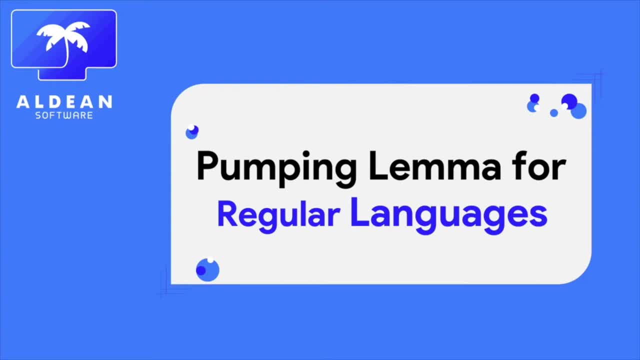 questions in an exam when they can be a lot of easy marks to pick up. From my experience, this is because lecturers tend to skip over some steps, assuming students will be able to make the. Now I'm here as a student to teach students. First, it's important to understand what the 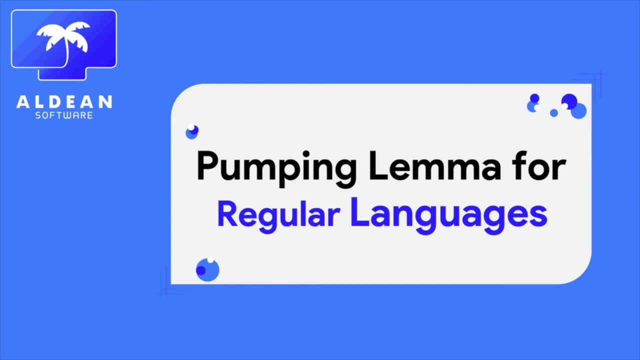 pumping lemma can and cannot be used for and how to use it. You can follow the timestamps in the description below to skip over this introduction and to move on to the worked examples. However, I would strongly recommend you listen to this whole thing for two reasons. 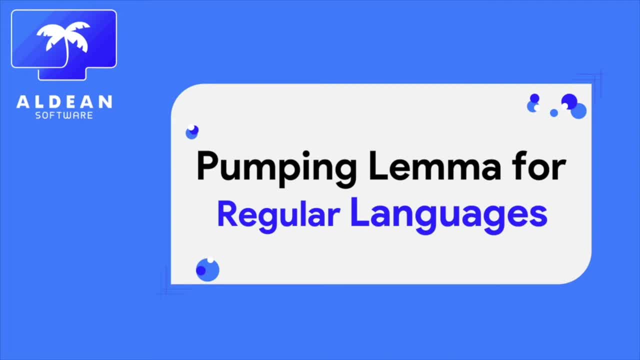 One, it's about when to and when not to use the pumping lemma. This is something many students often lose marks on. And two, even if it is something your lecturer or the other tutorials have mentioned, it is something that you can use. 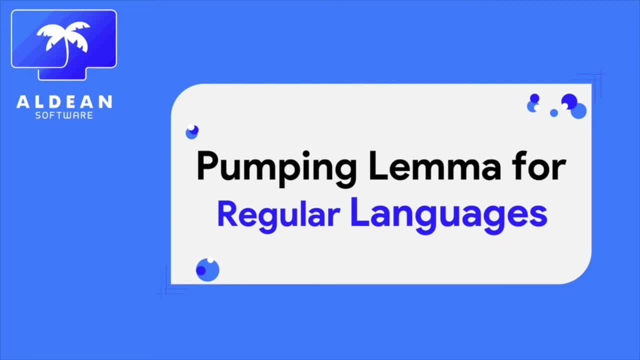 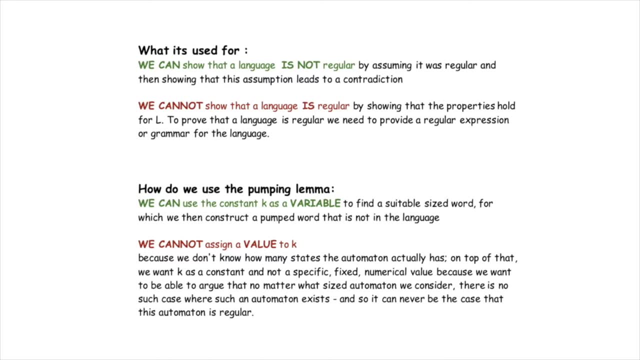 It is something students typically forget. The pumping lemma is a proof-by-contradiction method. Therefore we can use it to prove that a language is not regular. We do this by first assuming a language is regular and then showing that the properties of a regular language does. 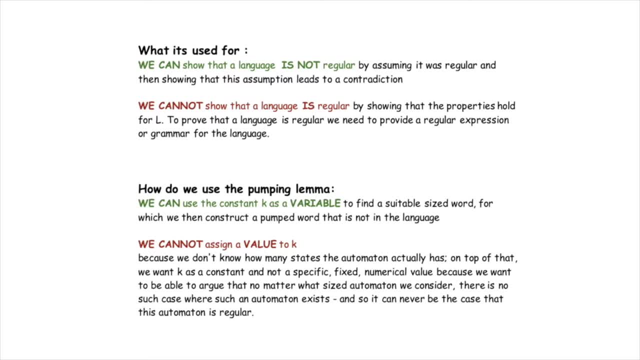 not hold when we pump up or pump down, and thereby finding a contradiction to the initial assumption. If, in an exam, you're asked to prove that a language is regular, showing that the properties hold for when we apply the pumping lemma to a word. 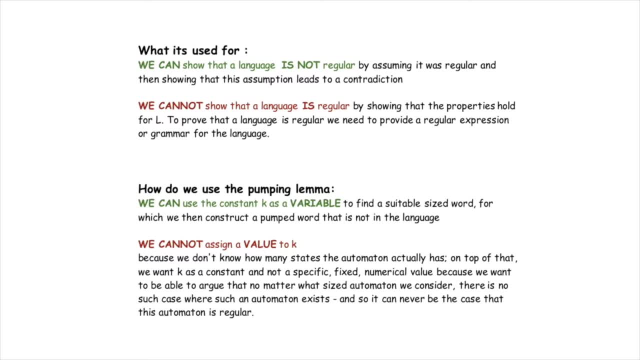 And that language is not enough to prove it. In this case you will need to find a regular language or grammar for the given language. To prove a language is not regular, we can use a constant k for the number of states as a variable meaning. we do not assign a. 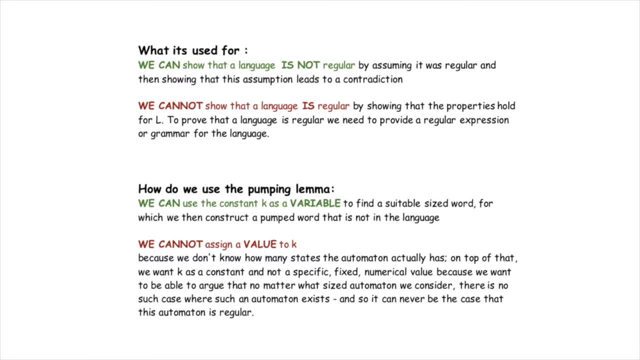 fixed value to k, We can use this variable to find a string that is greater than or equal to k in length. For this word we then construct a pumped word that is not part of the language and thereby prove by contradiction that the language must not be regular. We cannot assign. 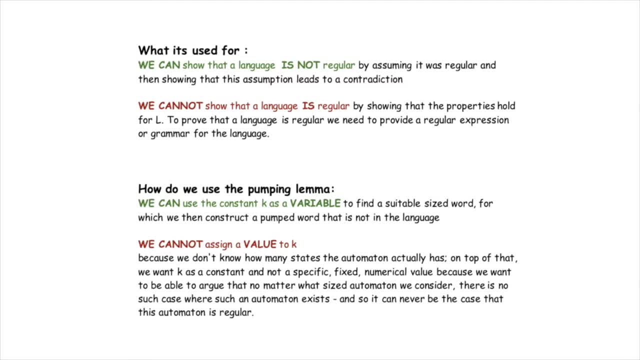 a value to k because we don't know how many states the automaton has. Remember, there can be several different automaton that describe the same language. We leave k as a constant to be able to argue that, no matter what the value of k is, there can never be a case where 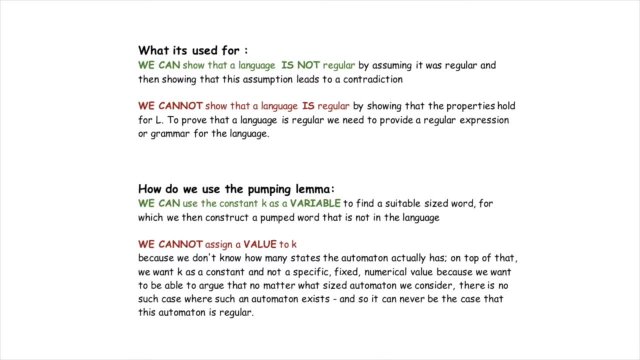 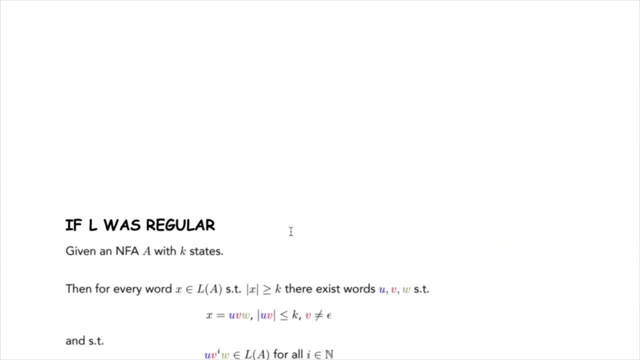 such an automaton exists for the given language. So there is no possibility for the given language to be regular. The general idea behind the lemma is given a non-deterministic finite automaton. so we know there is a finite automaton. we can use a general idea behind the lemma. 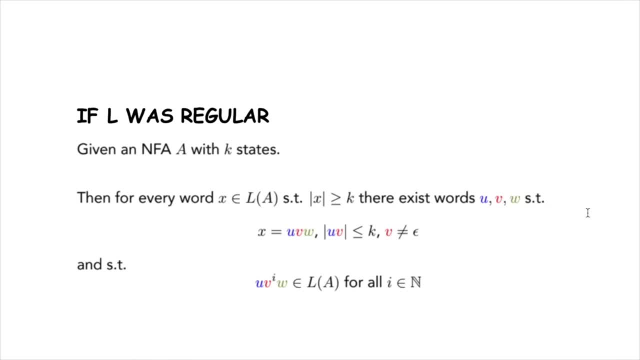 A finite number of states. If there are k states which may contain loops, the minimum length of any word x, which is a word within the language of the automaton A, would at least be the number of states, k or longer. For such a word x, you must be able to split. 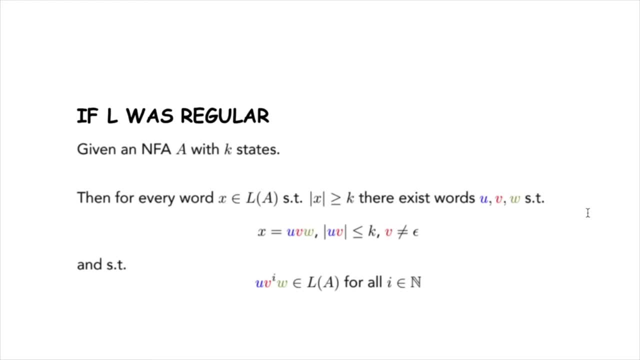 this word into three subwords- u, v and w, such that u is the first part of the word, v is the second part that contains the loop and therefore can be pumped up or down, and w is the end of the word. 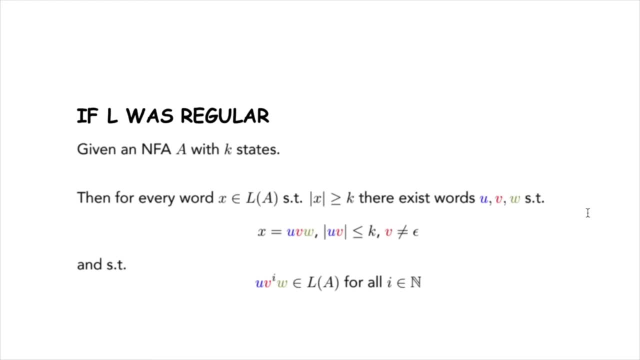 The first two subwords, u and v, together must contain the first k letters or less of the whole word x. The final condition is that the middle subword, v, which will be pumped, has to be at least one alphabet long. meaning v cannot be an empty word. 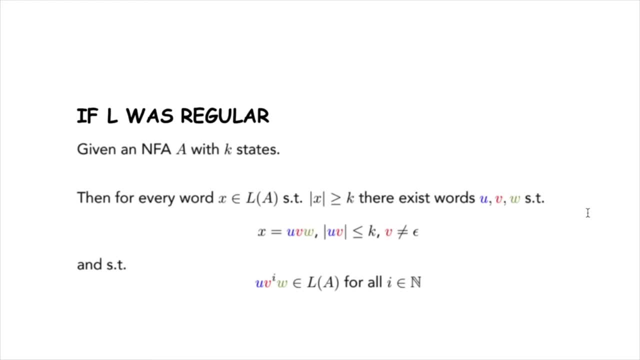 If the automaton A did indeed describe a regular language, then pumping the subword v would construct a new word that should also be a word in the language the automaton A describes. This means that raising v to the power of i would follow the properties of the language. 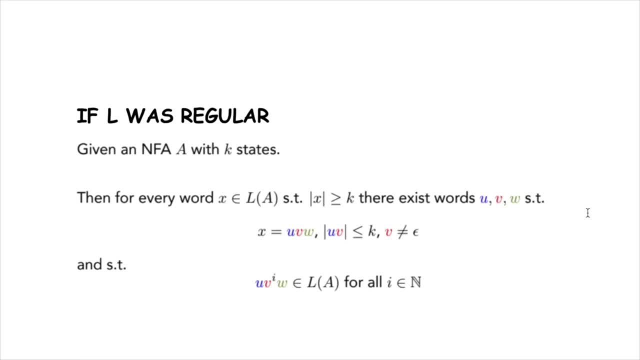 which is the number of states k and w. Note that i can be any natural number, including 0.. Now in the word composed of u, v and w, v is raised to the power of 1.. u v square w would mean we pumped the word and looped. 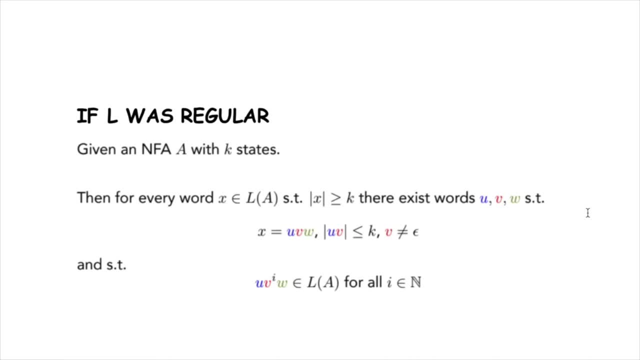 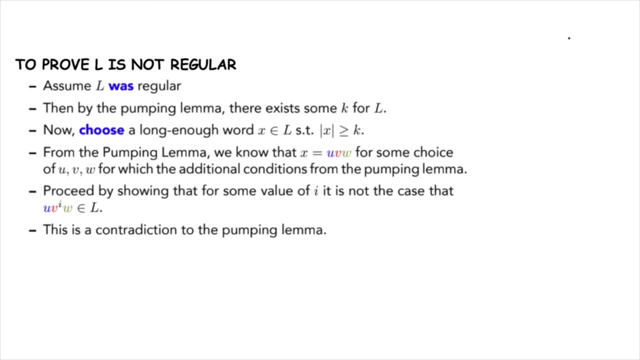 over a state. twice u v to the power 0 w would mean we pumped down and skipped the loop altogether. To prove that the automaton and the language of the automaton is not regular, we must first assume that the language is regular. 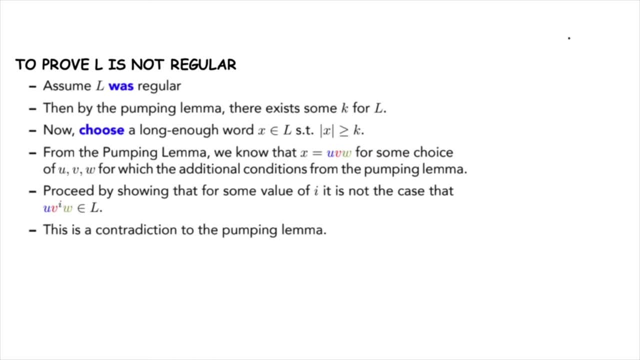 We then have to find out what the automaton is. We have a long enough word x, that is in the language L. What this means is that we have to define the word x in terms of k. The next step is to split the word in such a way that the first two subparts have to. 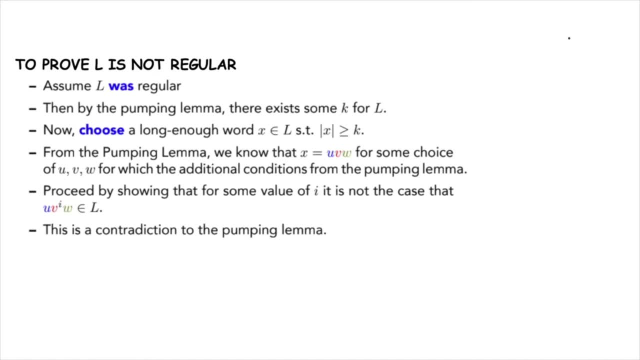 be within the first loop. The middle subword has to be at least one alphabet long. Finding a suitable word and splitting the word into its subpart takes some practice, but the more questions you practice you'll get a better hang of it. 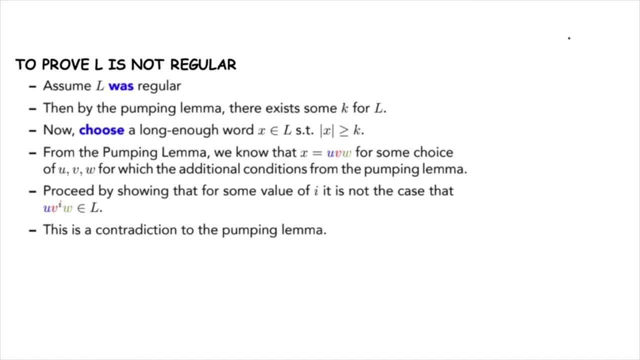 And I'll leave two questions with you to answer for yourself. There will be enough questions for you to answer. I'm going to show you another following video which you can use to check your answers. but make sure you do have an attempt first before you check them. 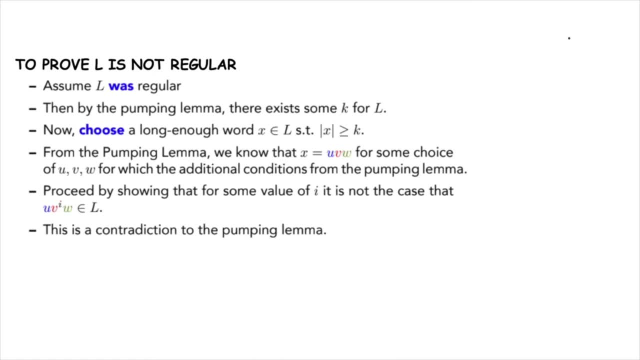 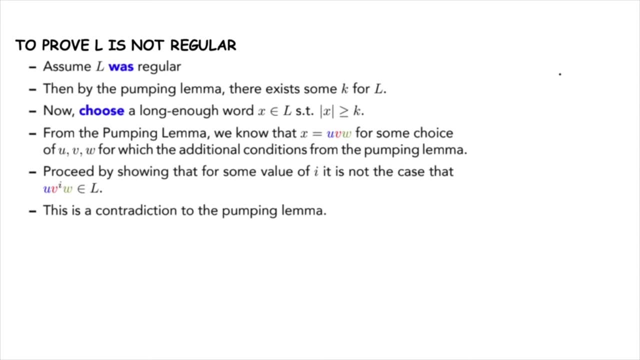 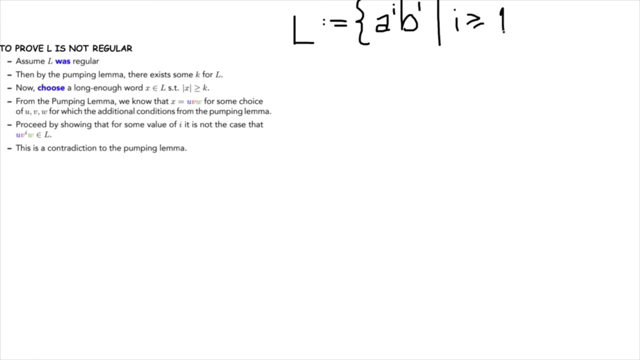 Remember: learning cannot be done passively. You have to actively take action. Make sure you do the questions yourself before you have a look at the answers. Here is the first example. Consider the following language: a to the i, b to the i where i is greater than or. 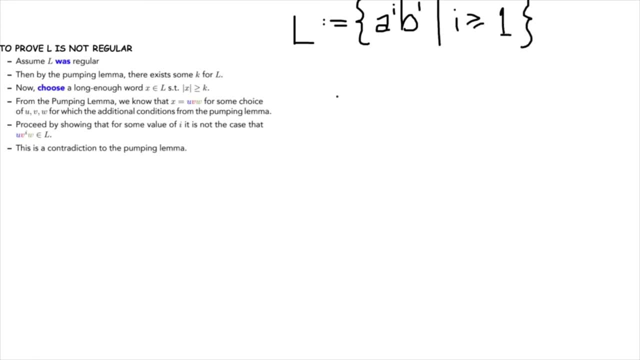 equal to 1.. This is essentially a block of a's followed by a block of b's of the same length. The first language that we'll learn is the following: a to the i. b to the i where i is greater than or equal to 1.. 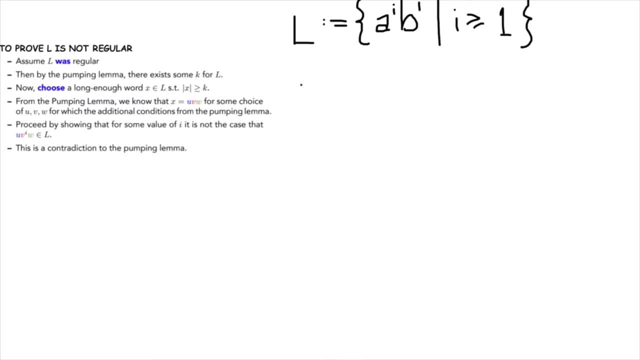 This is essentially a block of a's followed by a block of b's of the same length. Assuming this language is a regular language, there will be a finite automaton to describe this language with k states. Now to choose a word: x. we could say a to the power, k, b. 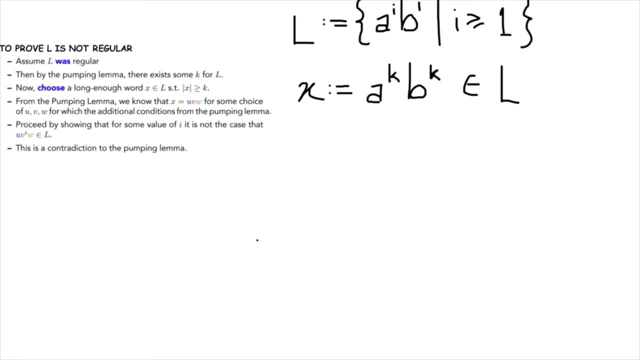 to the power. k is a word in this language. If we imagined an automaton for such a word, the first loop would be after the first a. This word, x, is greater than k in length because it has two blocks of length, k. Now, if we were to split this word into three subparts, 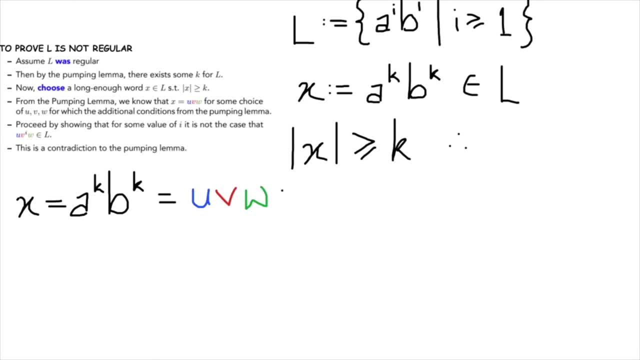 where u and v have to be within the first k letters or less. so the word x, which is a to the k, b to the k, will be split, so that some of the k a's and the rest of the b's will have to be the tailing subword w, so that u will be an arbitrary number of a's. 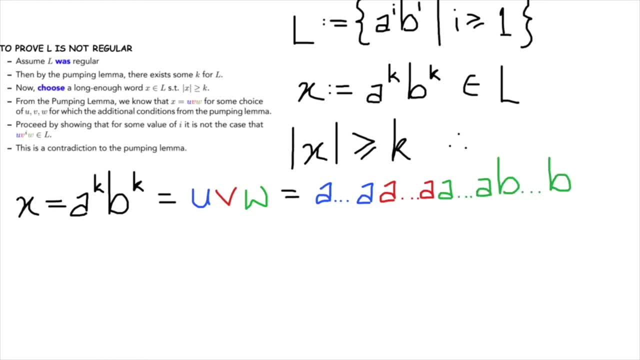 and v will be another arbitrary number of a's. So finally, a to the k, b to the k is split into three parts: a to the i, a to the l and the remaining a's, which is total number of k minus i, plus l and kb's. This is how we split a to the k, b to the k into u, v and w. 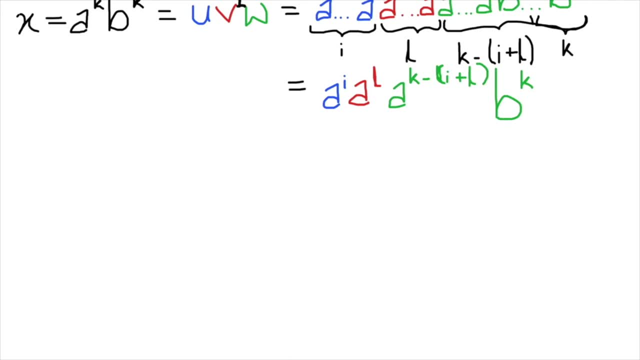 Here the original word x is split into u, v to the 1 and w. When we pump up the word once more we have u, v square and w. We now have two blocks of a to the l, because a to the l is the middle. 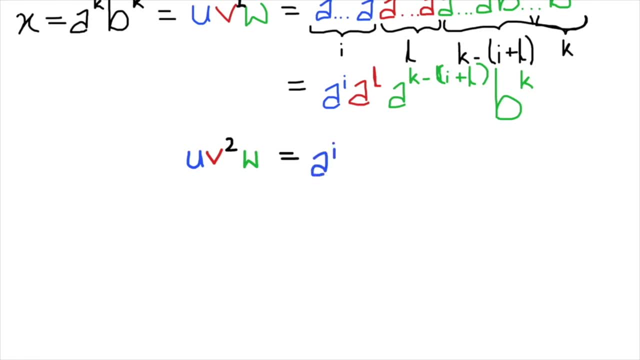 subword v, which we pumped up from v raised to 1 to v raised to 2.. This new pumped word is composed of: a to the i, a to the l twice and a to the k minus i, plus l in brackets. b to the k. 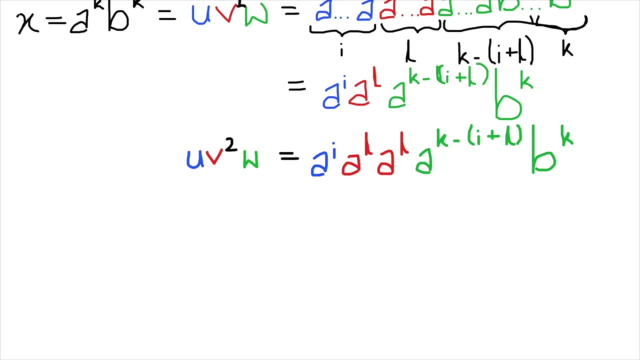 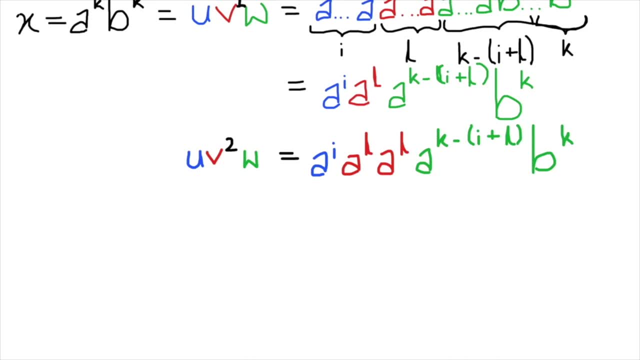 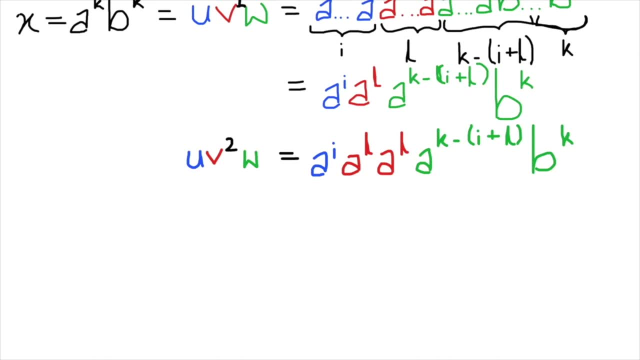 saw it when I expanded all the indices. When we expand k minus i plus l, we get k minus i and minus l. Negative indices mean that we can divide the a's by a to the l and a to the i. Simply put, we can cross off a to the i, a to the l, with the i plus l in the brackets. After simplification, this: 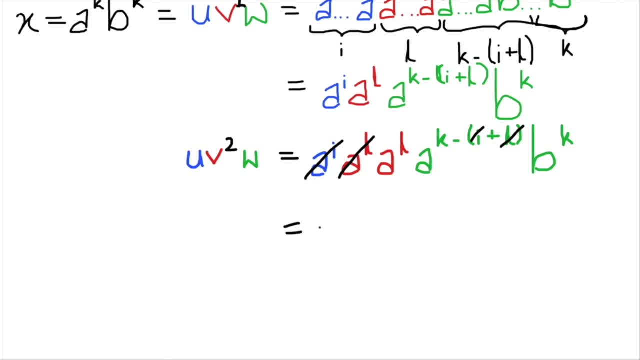 leaves us with the new pumped up word: uv squared w to be a to the k plus l, b to the k. This word is not the same as a to the k, b to the k, a to the k plus l, b to the k is not a word in the language. 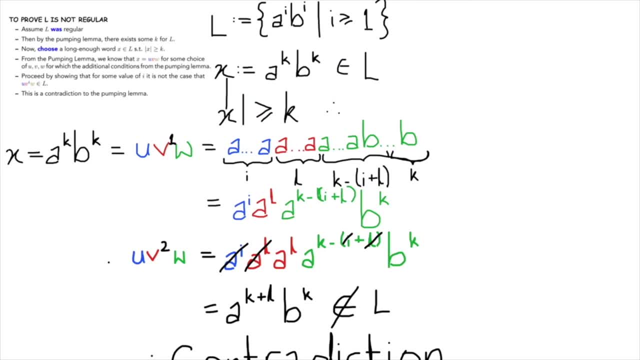 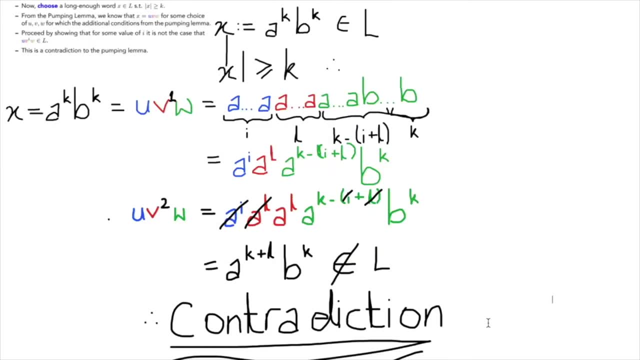 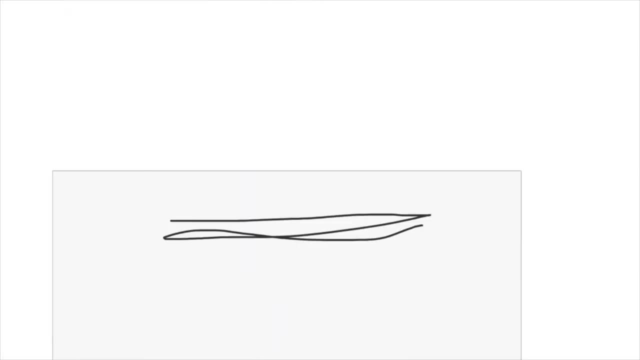 This is a contradiction. Therefore, we have proved by the pumping lemma that this language cannot be regular. I hope this explanation was easy to follow through with. If you haven't understood it yet, I'll be going through another example. Even if you have understood it, I would advise you to still have a look at how we solve. 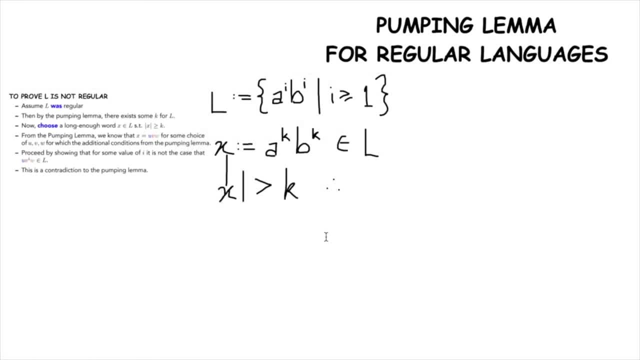 another example to further grasp the idea. There will also be two questions at the end of this video which I would like for you to have a go at to test yourselves on whether you have understood it. The answers will be given in another video. Consider the following language: x, x, r, such that x. 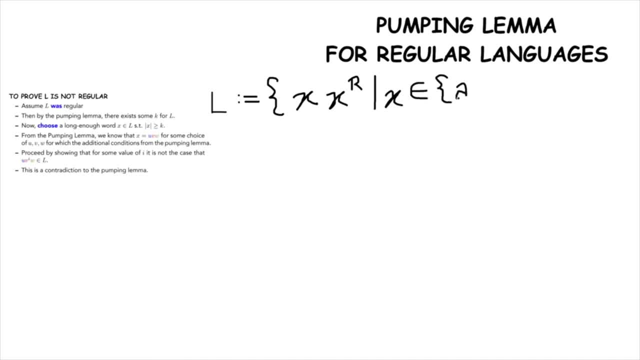 is a word composed of a's and b's. The Kleene star means that this includes the empty word. If it were a plus, it would have to be any word over the alphabet a- b that is at least one alphabet long. This is essentially the language. 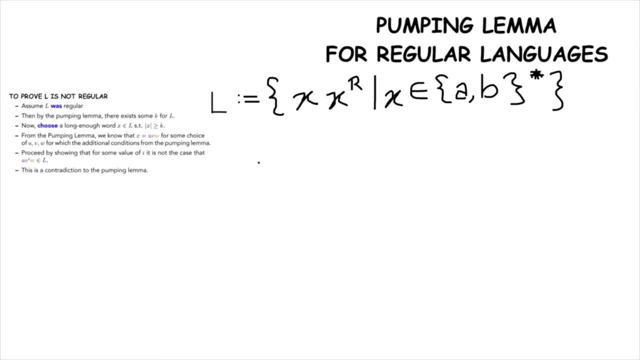 consisting of all, even palindromes. It's all, even palindromes because the subword x is attached to its reverse word. The capital r as a superscript means the reverse of the word x. If x has three alphabets, joining it with its reverse will give six alphabets. If x had two, joining it with its. 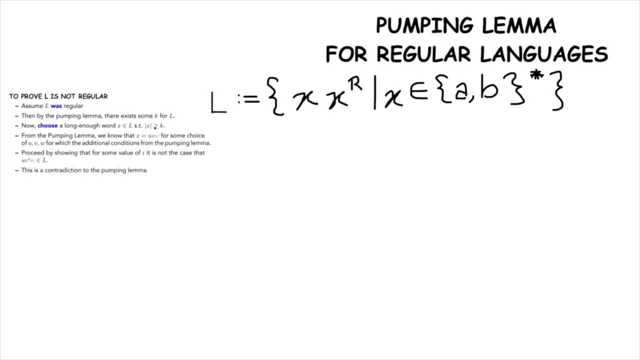 reverse gives you four alphabets. In any case, you will always get a palindrome of even length. A long enough word that we notice in this language could be x equals a to the power k b, followed by its inverse b, a to the power k. Again, assuming this language is regular, there must exist an. 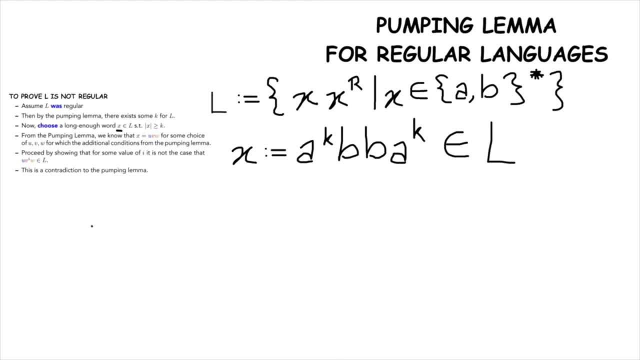 automaton function that can be used to calculate the value of any of the three alphabets If x is for it, and therefore there must exist some k for this language. L And this word, x equals a to the k, b, ba to the k- can be split into three subparts: u, v and w. Because u and v has to be within the. 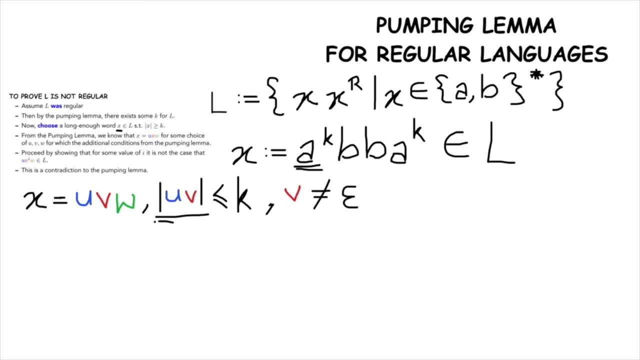 first k alphabets, u and v, has to be within the first k a's. Therefore, again, u will be an arbitrary block of a's less than the length of k. v will be another arbitrary length of a's less than k. w will be the remaining k a's followed by b, b, a to the power, k, So u, v to the power 1. 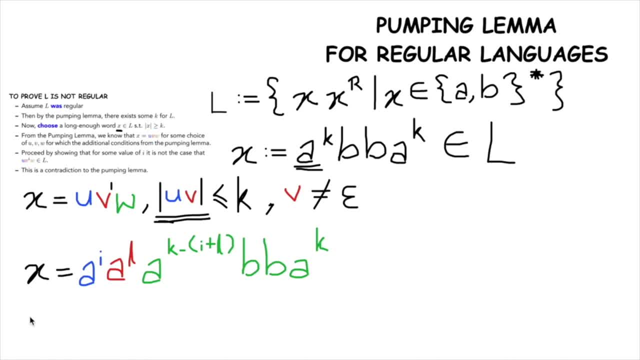 w is a to the i, a to the l, a to the k, minus i, plus l b b, a to the k. If we pump this word up to get u v squared w, u v squared, w will equal to a to the i, a to the l. 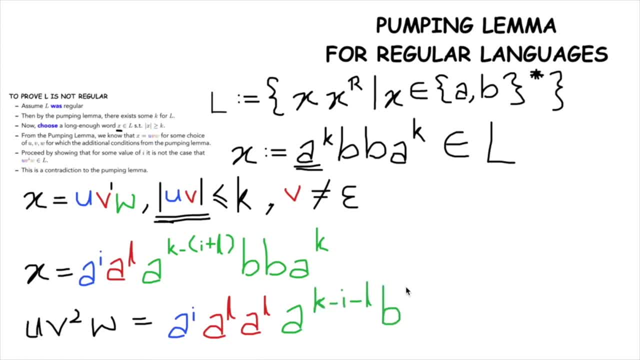 a to the k minus i, plus l b b a to the k. Twice a k minus i, minus l b b a to the k. We can again cross off a to the i with minus i and a to the l with minus l, Leaving us with a to the k, a to the l b b a to the k. 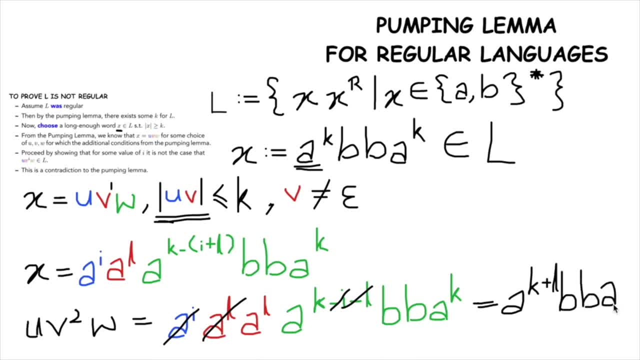 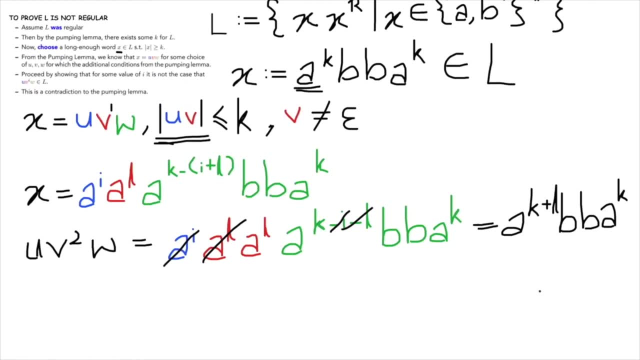 which we can simplify to: a to the k plus l b b. a to the k. a to the k plus l b b. a to the k is not the same as a to the k, b, b, a to the k. therefore, a to the k plus l b b. a to the k is.